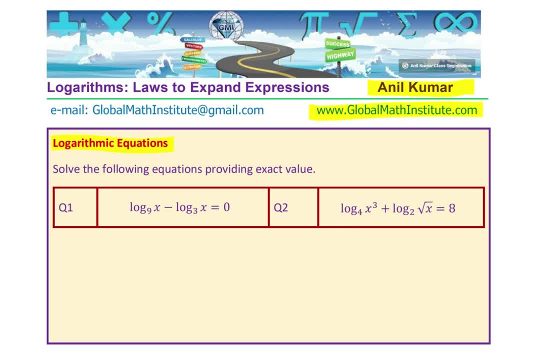 base 4 of xq plus log to the base 2 of x. square root of x equals to 8.. I would like you to pause the video, answer the question and then look into my suggestions. In case you need my help, you can always email on the address given. 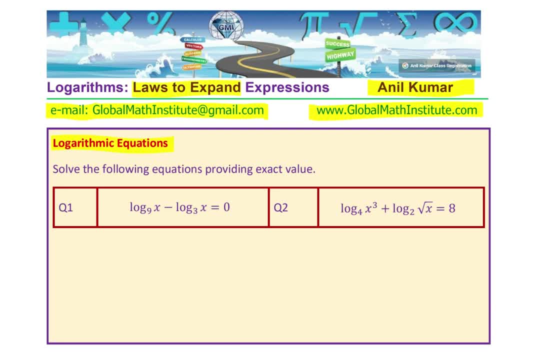 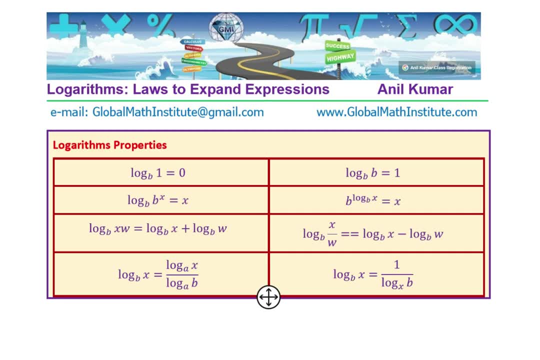 Let us explore laws of exponents and then see how can we change the base and then solve these equations. Well, here is a reminder of the logarithmic properties or laws, And change of base formula is given right there. Perfect. So basically, if you want to change, 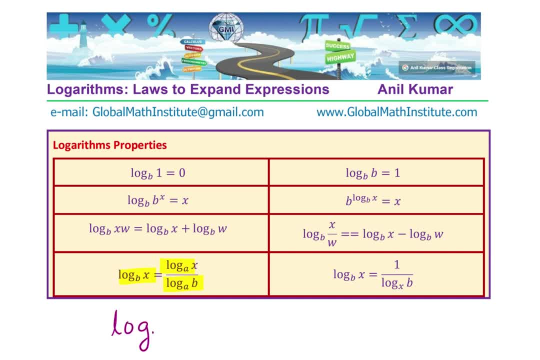 the base. let me rewrite this formula slightly bigger: Log to the base p of x, to something like p, So you can write in the numerator: log to the base e of x and then divide by log to the base a of p. Then you get the same base. You get the idea And now, using the 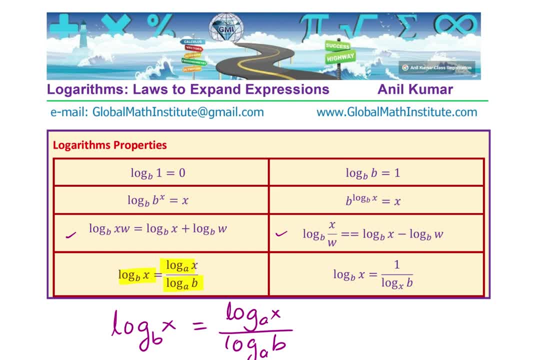 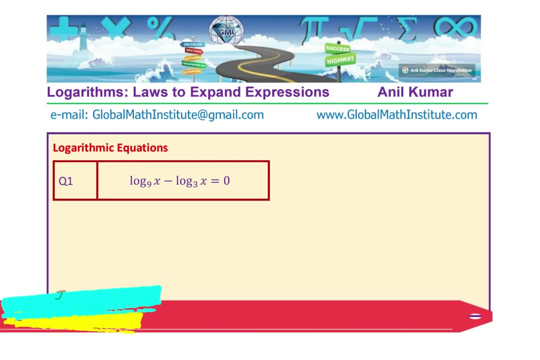 other properties of logarithms, you could solve the logarithmic equation. So with that I would like you to try and solve this equation and then check. with my solution Perfect. So the equation is: log to the base 9 of x minus log to the base 3 of x equals to 0. 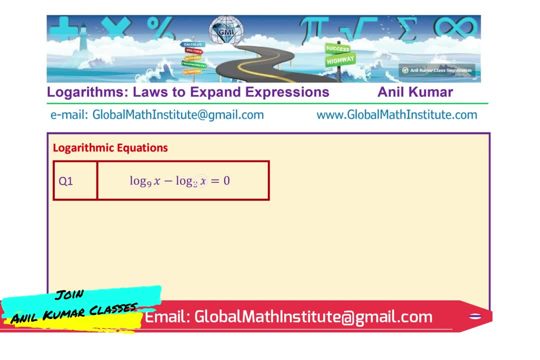 Since the base is different, we cannot really write x over x or something like this. How do we change the base Using the formula we have: log to the base 9 of x. We would like to change it to 3.. So we can write this as log to the base 3 of x, divided by log to the: 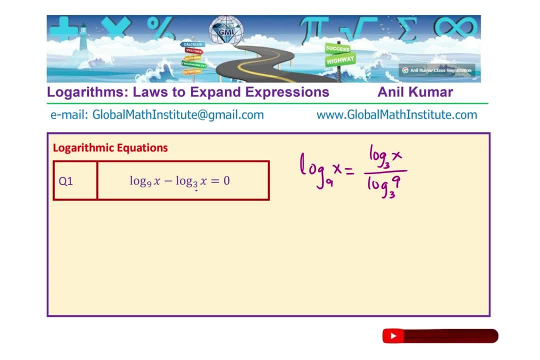 base 3 of 9.. Now, what is the denominator? 9 can be written as 3 square, right? So I could write this as log to the base 3 of x, over log to the base 3 of 3 square, And that. 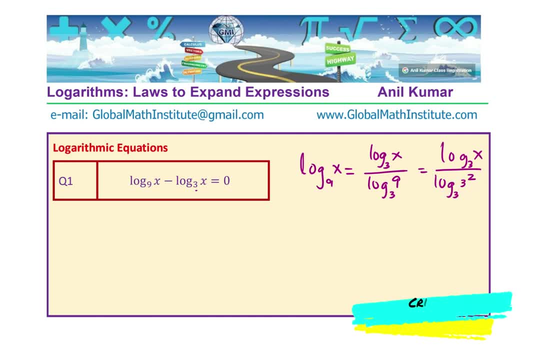 gives you an idea that this denominator should be not 2, right, So we can rewrite this expression. So now getting back to the equation, So we have this equation, which is log to the base 9 of x, minus log to the base 3 of. 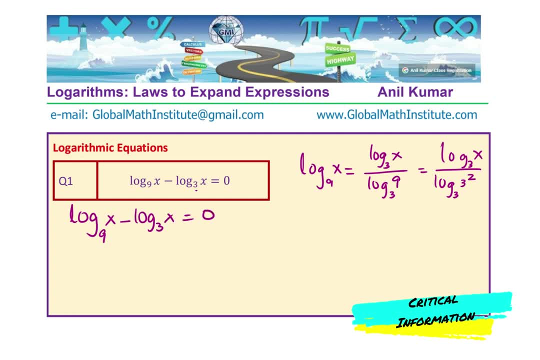 x equals to 0.. What should we do? We will change the base from 9 to 3.. And then what do we get? We get log to the base 3 of x over this expression. Now, what is log to the base? 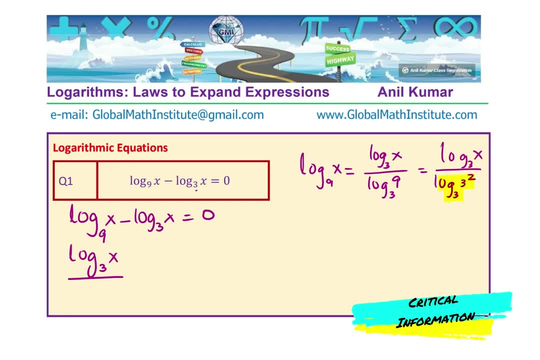 3 of 3 square. It is just the number 2, right? So I am writing 2 here. So I am writing 2 here for that, And then we will rewrite the next term, which is minus. log to the base. 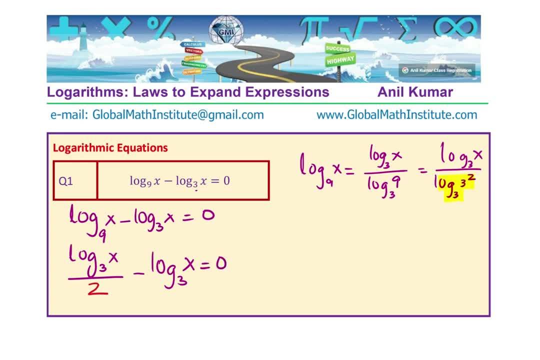 3 of x equals to 0.. Do you get it How we got from here to this place? The base log to the base. 3 of 3 square is equal to 2.. So we substituted that correct. So now clearly. 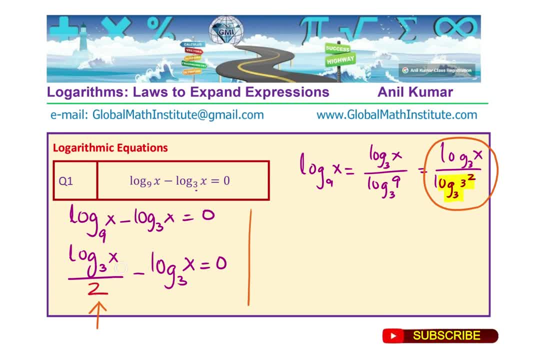 what do we have? We have 2 in the fraction. Let us multiply each term by 2, okay. So if we multiply each term with 2, we get what We get. log to the base 3 of x minus 2. log to the base 3 of x. 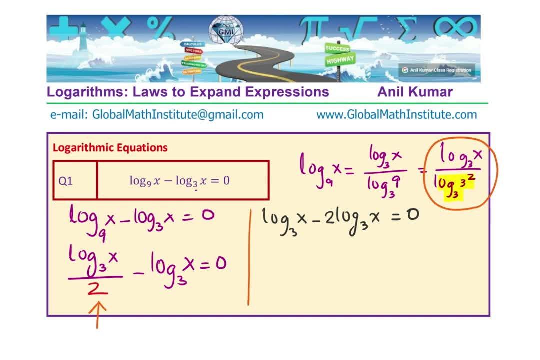 equals to 0. I could have taken it to the other side also. Now, what is log to the base 3 of x minus 2 log to the base 3 of x? They can be combined. That gives me minus log to. 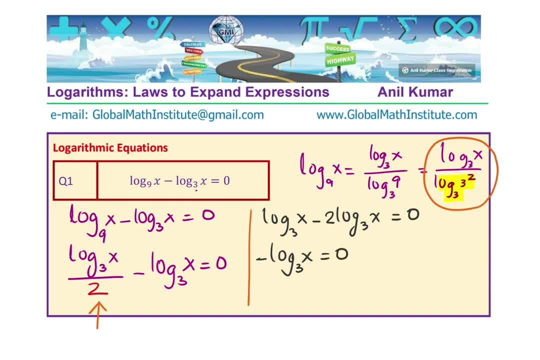 the base 3 of x equals to 0.. Well, that gives me log to the base 3 of x equals to 0, and now we can find the value of x. Can you write down the solution? Well, clearly it means. 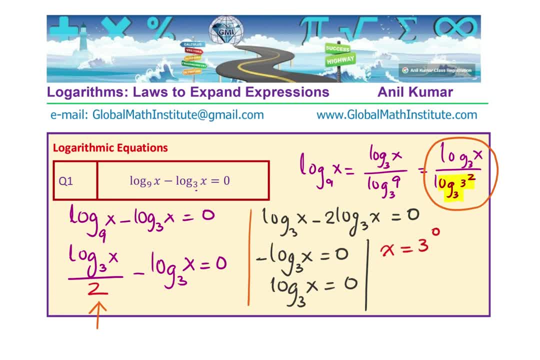 x is equal to 3 to the power of 0, and anything to the power of 0 is 1.. And therefore we have our answer, which is x equals to 1.. It's a good idea to check your result right. So if you substitute log to the base 9 of 1 minus log to the base, 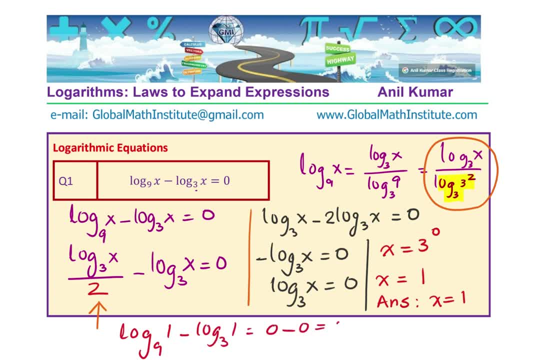 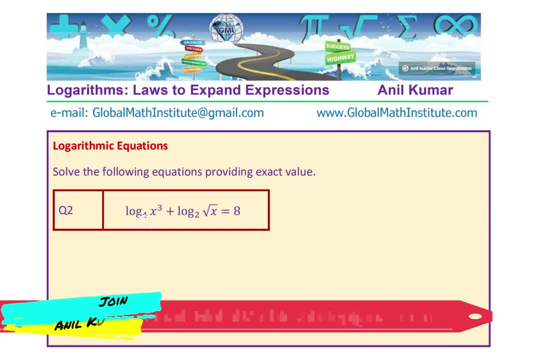 Well, you already know the equation, Question number 2, which is log to the base 4 of x cubed plus log to the base 2 of x. squared over, x equals to 8.. Well, we need to change this base to 2, right, So let's do that, So we can rewrite this equation as log to. 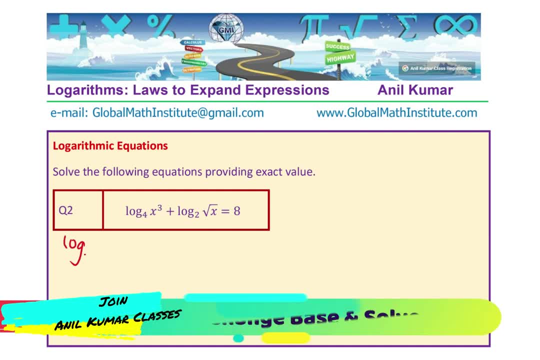 the base Instead of 2, instead of 4, I am writing 2 x cubed, so I have changed the base to 2, divided by log to the base 4 of x cubed, base 2 of 4, right. And then we have plus log to the base 2 of square root of x, which is x to the 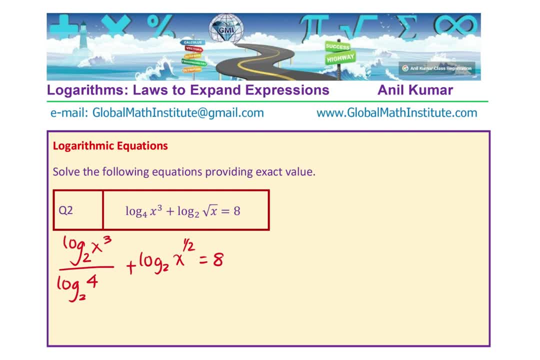 power of half, and that is equal to 8.. Now, log to the base 2 of 4 is 2, right, Because 4 is 2 squared. yes, so I could write this as log to the base 2 of x cubed over 2, perfect, plus that is. 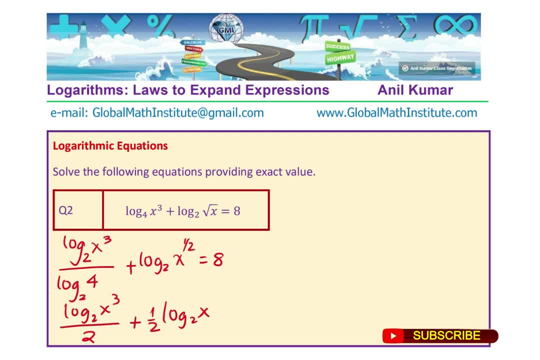 half of log to the base 2 of x equals to 8.. The numerator here is 3 times log to the base 2 of x, right? So we could write this as 3 times and there's 2 in the denominator: log to the base 2. 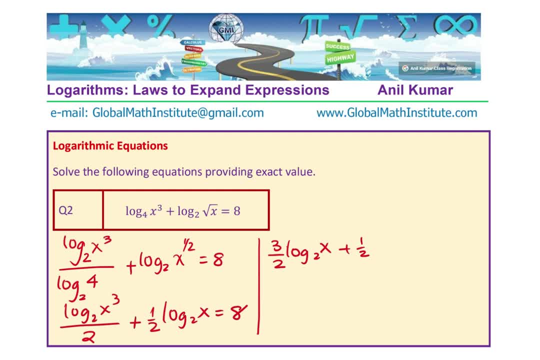 of x plus half of log to the base 2 of x equals to 8.. So we can combine these terms: log to the base 2 of x plus half of log to the base 2 of x equals to 8.. x common. we get 3 over 2 plus half equals to 8, and 3 over 2 plus half is 1 right. 4 over 2 right. 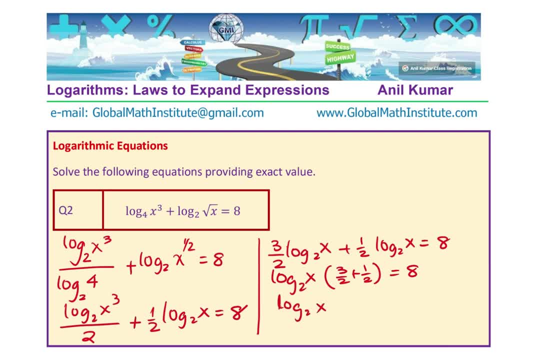 so it is log to the base 2 of x, and this is 3 plus 1, 4. 4 over 2, which is 2, equals to 8. so we have log to the base 2 of x, equals to 8 over 2, which is 4, and from here you can find what x is.